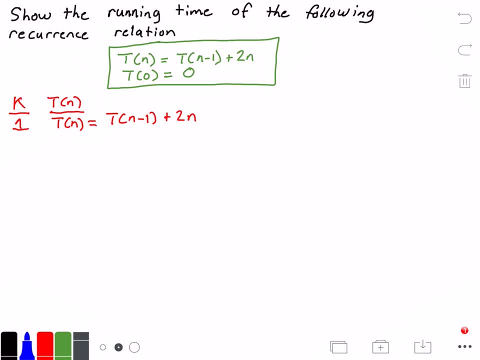 figure out what t of n minus 1 is, and we can do that by substituting n for n. in our, in our recursive case, We're going to substitute n n minus 1, and so let me show you, guys, what that means. So t of n minus 1 now is going to be equal to t of n minus 1 minus 1 plus 2 times n minus 1. and if we 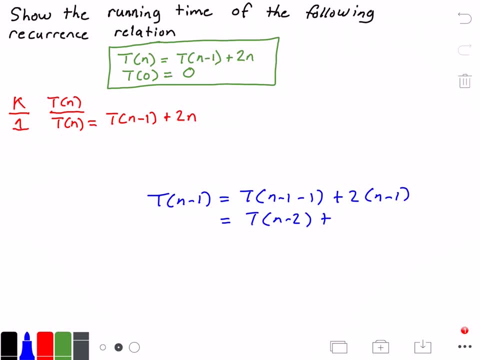 simplify this. we get t of n minus 2 plus 2 times n minus 2.. Okay, so this means that we can substitute. now we can substitute n for t of n minus 1. we can substitute in: t of n minus 2 plus 2 times n. 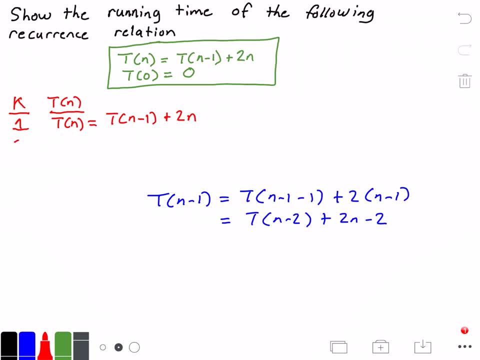 minus 2.. So now this is our second step. So k is equal to 2 and our function t of n is equal to t of n minus 2 plus 2 times n, minus 2 plus 2 times n. All right, so I'm going to go ahead and 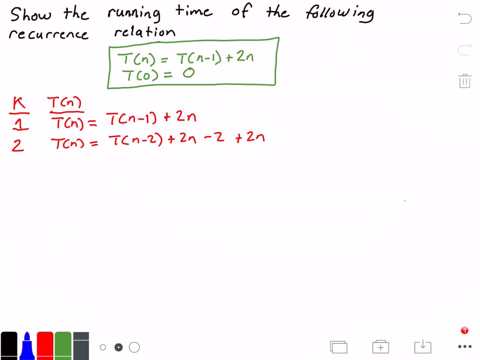 write this down. So I'm going to go ahead and write this down, So I'm going to go ahead and erase this down below and I'm going to kind of explain exactly what we did here. So our function t of n minus 1 has now become t of n minus 2, plus 2 times n minus 2, and then we've added the 2 times. 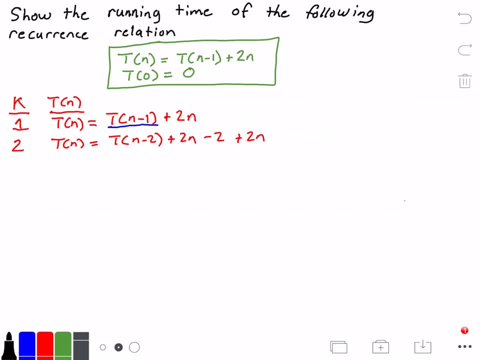 n here. All right, okay. so I want to simplify this a little bit. So this is going to be equal to t of n minus 1 plus 2 times n minus 2 plus 2 times n minus 2.. So I'm going to go ahead and 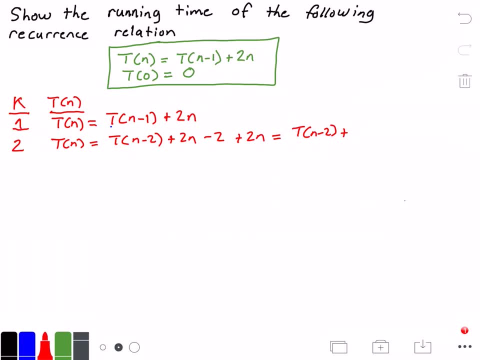 t of n minus 2 plus 2 times 2 times n minus 2.. Okay, all right. so now we need to figure out what t of n minus 2 is, and to do that, we're going to basically do the same thing, So we get. 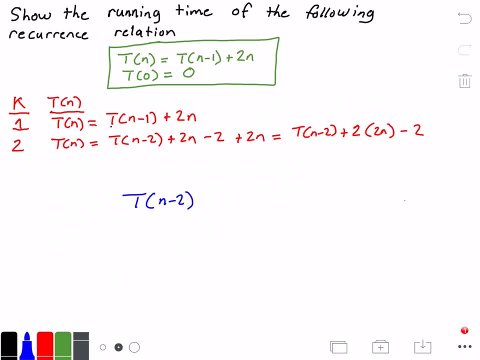 t of n minus 2 plus 2 times n minus 2 plus 2 times n minus 2 plus 2 times n minus 2.. is equal to t of n minus 2 minus 1 plus 2 times n minus 2.. And if we simplify this, we get t of n. 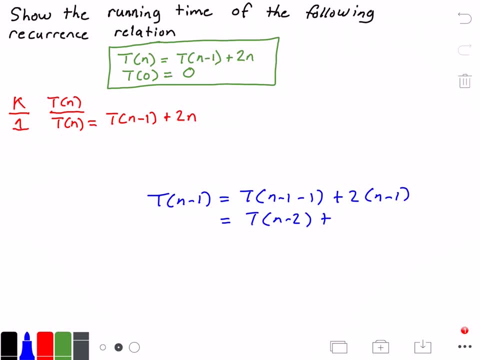 simplify this. we get t of n minus 2 plus 2 times n minus 2.. Okay, so this means that we can substitute. now we can substitute n for t of n minus 1. we can substitute in: t of n minus 2 plus 2 times n. 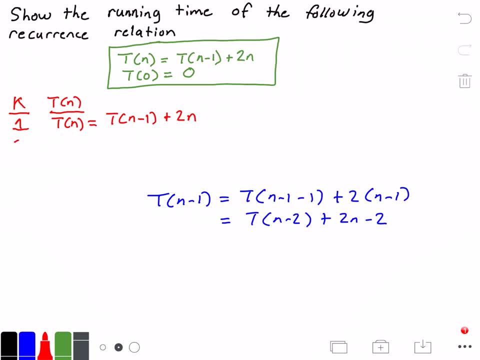 minus 2.. So now this is our second step. So k is equal to 2 and our function t of n is equal to t of n minus 2 plus 2 times n, minus 2 plus 2 times n. All right, so I'm going to go ahead and 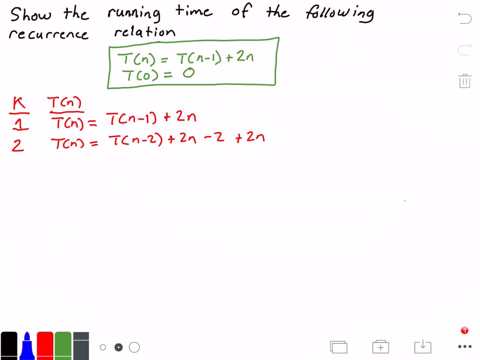 write this down. So I'm going to go ahead and write this down, So I'm going to go ahead and erase this down below and I'm going to kind of explain exactly what we did here. So our function t of n minus 1 has now become t of n minus 2, plus 2 times n minus 2, and then we've added the 2 times. 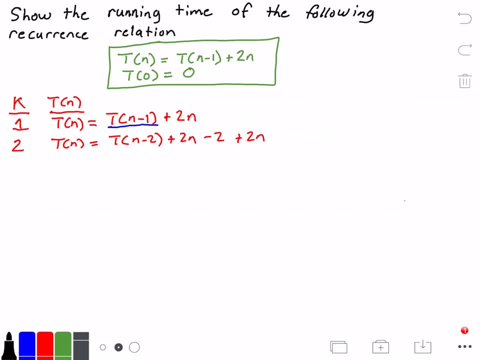 n here. All right, okay. so I want to simplify this a little bit. So this is going to be equal to t of n minus 1 plus 2 times n minus 2 plus 2 times n minus 2.. So I'm going to go ahead and 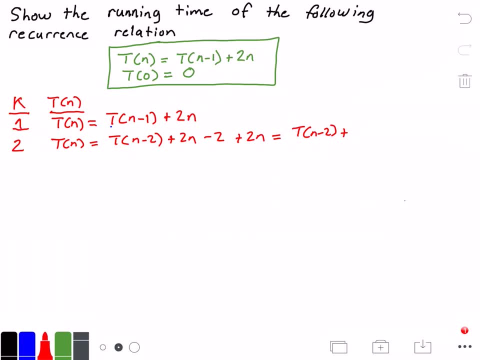 t of n minus 2 plus 2 times 2 times n minus 2.. Okay, all right. so now we need to figure out what t of n minus 2 is, and to do that, we're going to basically do the same thing, So we get. 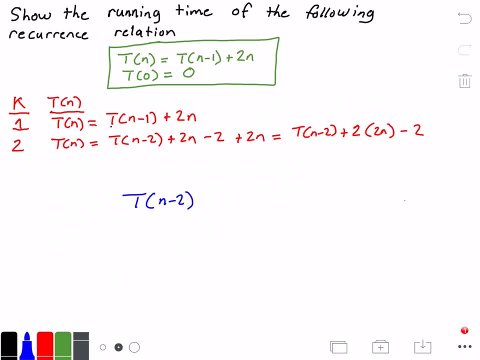 t of n minus 2 plus 2 times n minus 2 plus 2 times n minus 2 plus 2 times n minus 2.. is equal to t of n minus 2 minus 1 plus 2 times n minus 2.. And if we simplify this, we get t of n. 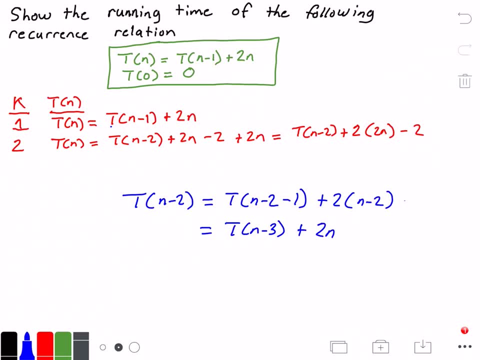 minus 3 plus 2 times n minus 4.. Okay, so now k is going to equal 3 and our function t of n is going to be equal to t of n minus 3 plus 2 times n minus 4.. All right, and then we're going to add in 2 times 2. 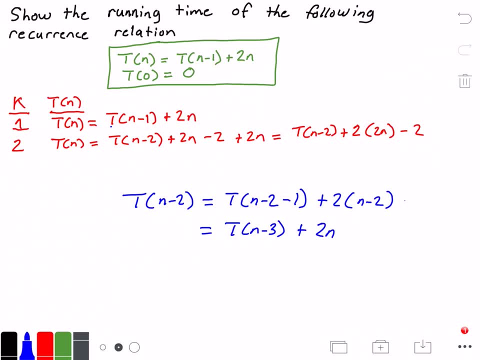 minus 3 plus 2 times n minus 4.. Okay, so now k is going to equal 3 and our function t of n is going to be equal to t of n minus 3 plus 2 times n minus 4.. All right, and then we're going to add in 2 times 2. 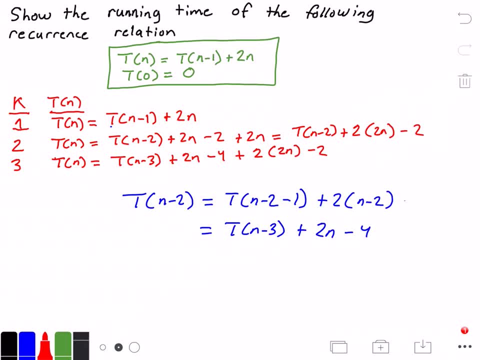 times n minus 2.. All right, so let's go ahead and erase this here and let's kind of show what we did again. so now t of n minus 2 became t of n minus 3 plus 2 times n minus 2 plus 2 times n minus 3 plus 2 times n minus 2!. Okay, so now we're going to. 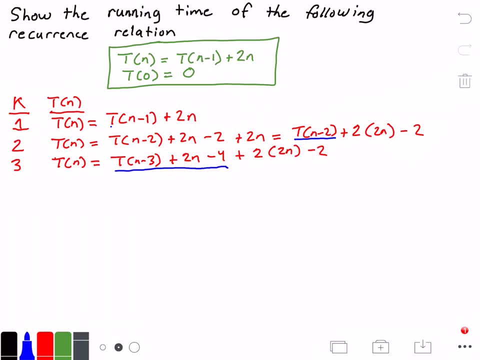 times n minus 4.. And then we needed to add 2 times 2 times n minus 2.. And we did that here 2 times 2 times n minus 2.. All right, Okay, And so we're going to keep doing this until we see. 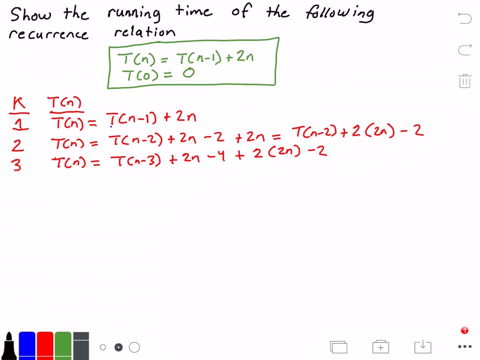 a pattern. But I don't see a pattern yet, So let me go ahead and simplify that equation that we just now wrote. So we get t of n minus 3 plus 3 times 2 times n minus 4 minus 2.. I still don't. 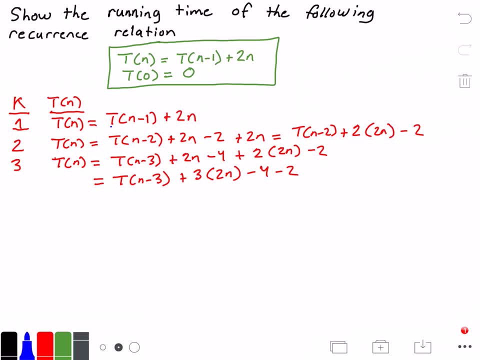 see a pattern. So let's go another step here And let's solve for t of n minus 3.. So t of n minus 3 is going to be equal to t of n minus 3 minus 1 plus 2 times n minus 3.. 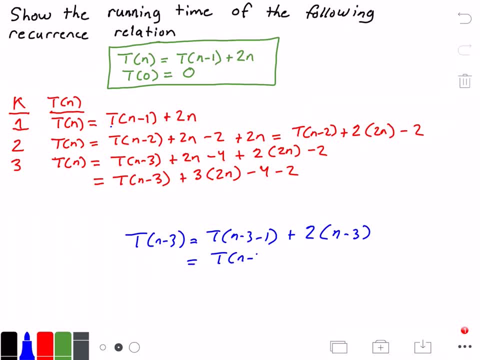 And if we simplify this, we get t of n minus 4 plus 2 times n minus 6.. And so now our k will equal 4.. And our function, t of n, will be equal to t of n minus 4 plus 2 times n minus 6 plus 3 times. 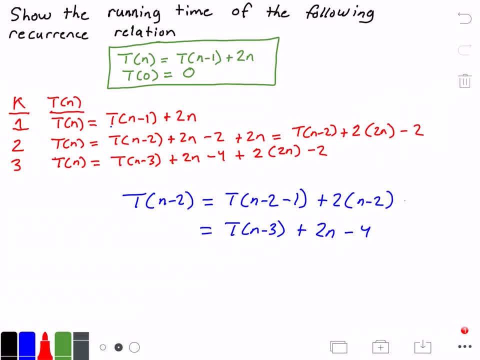 times n minus 2.. All right, so let's go ahead and erase this here. And that's kind of show what we did again. So now t of n minus 2 became t of n minus 3, plus 2 times n minus 4.. And then we needed to add 2 times 2 times n minus 2.. And we did that here. 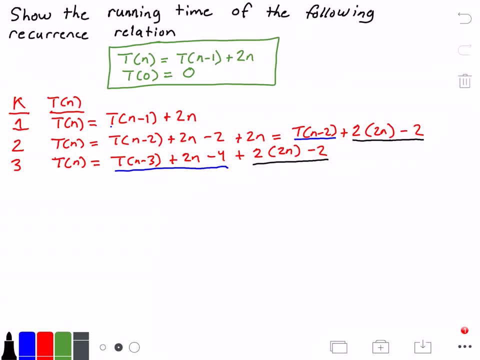 2 times 2 times n minus 2.. All right, Okay, And so we're going to keep doing this until we see a pattern. But I don't see a pattern yet, So let me go ahead and simplify that equation that we 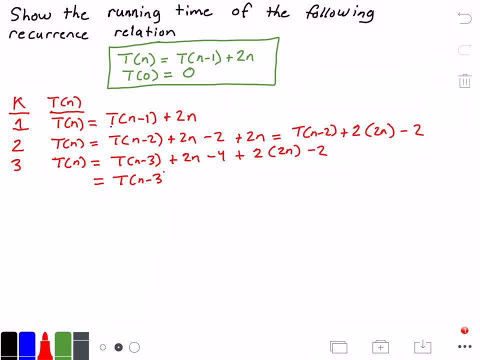 just now wrote. So we get t of n minus 3 plus 3 times 2 times n minus 4 minus 2.. I still don't see a pattern, So let's go another step here And let's solve for t of n minus 3.. 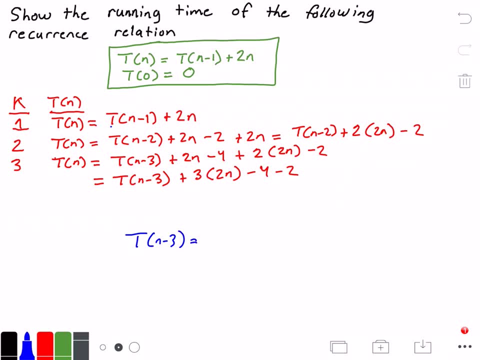 So t of n minus 3 is going to be equal to t of n minus 3 minus 1 plus 2 times n minus 3.. And if we simplify this, we get t of n minus 4 plus 2 times n minus 6.. And so now our k will. 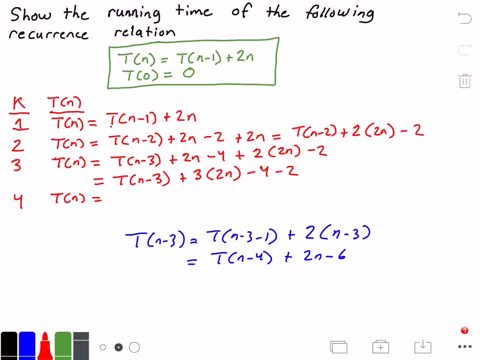 equal 4.. And our function t of n will be equal to t of n minus 4 plus 2 times n minus 6 plus 3 times 2 times n Minus 4 minus 2.. Okay, So I'm going to erase that what we did below, And let's simplify this. 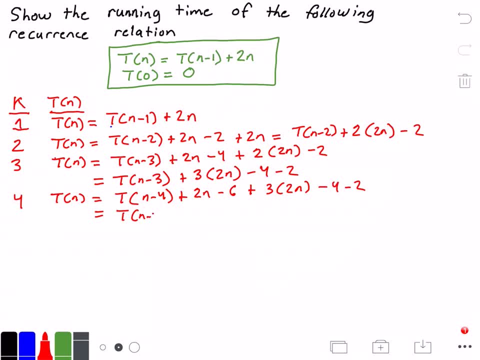 equation. So we get t of n minus 4 plus 4 times 2 times n minus 6 minus 4 minus 2.. All right, So now I do see a pattern, So let's take the equations and rewrite them below. So we're going to take 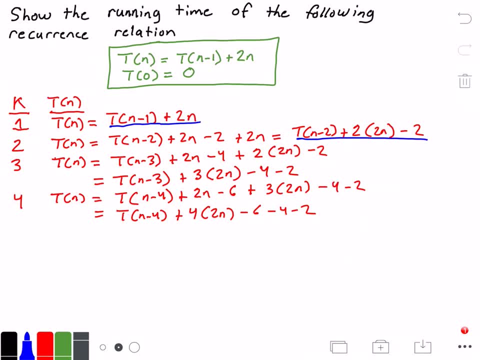 that first equation here. We're going to take this equation here. We're going to take this equation here and this last one here, All right, So when k is equal to 1, we get t of n minus 1 plus 2 times. 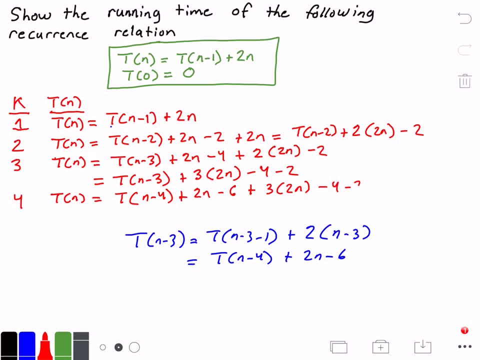 2 times n Minus 4 minus 2.. Okay, So I'm going to erase that what we did below, And let's simplify this equation. So we get t of n minus 4 plus 4 times 2 times n minus 6 minus 4 minus 2.. All right, So. 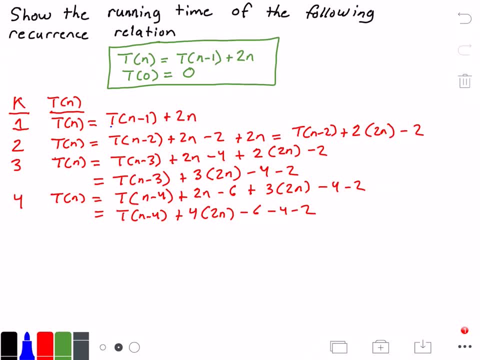 now I do see a pattern, So let's take the equations and rewrite them below. So we're going to take that first equation here, We're going to take this equation here, We're going to take this equation here and this last one here. All right, So when k is equal to 1, we get t of n minus 1 plus 2 times. 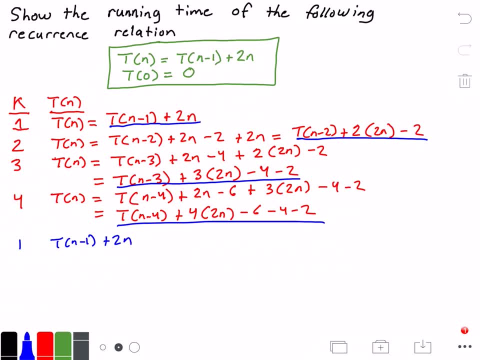 n, And I'm doing this so you guys can see the pattern. I do see a pattern now. When k is equal to 2, we get t of n minus 2.. Plus 2 times 2 times n minus 2.. Okay. And when k is equal to 3, we get t of n minus 3 plus 3 times 2. 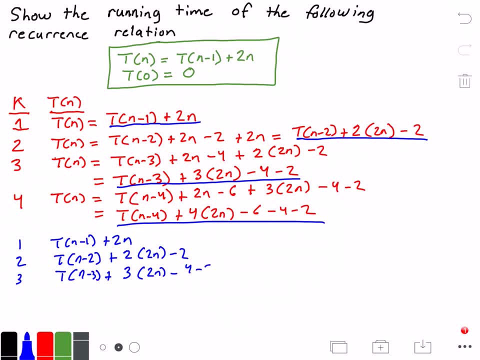 times n minus 4 minus 2.. And when k is equal to 4, we get t of n minus 4 plus 4 times 2 times n minus 6 minus 4 minus 2.. Okay, So I'm going to erase everything that we did before And hopefully now you guys can see a. 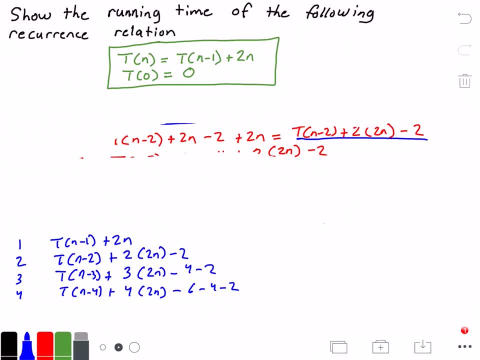 pattern as well. If not, I will try my best to explain. Okay, All right. So here we have our k iterations and we have our function t of n. All right, So when k is equal to 1, we get t of n. 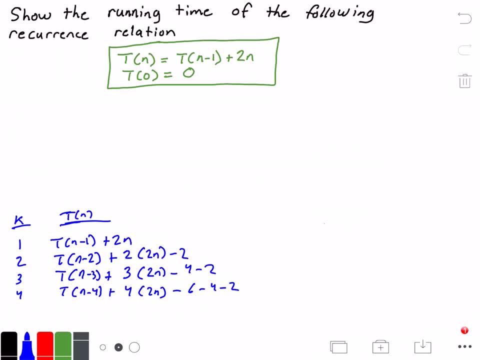 minus 1.. When k is equal to 2, we get t of n minus 2.. When k is equal to 3, we get t of n minus 2.. When k is equal to 3, we get t of n minus 3.. And when k is equal to 4, we get t of n minus 4.. So 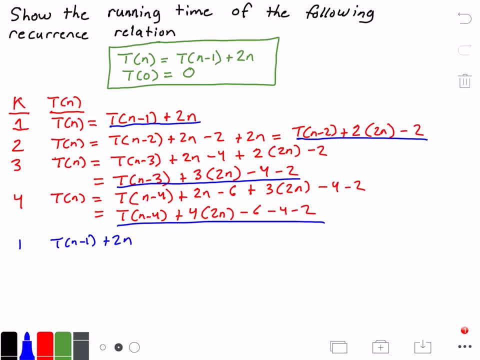 n, And I'm doing this so you guys can see the pattern. I do see a pattern now. When k is equal to 2, we get t of n minus 2.. plus 2 times 2 times n minus 2.. Okay. And when k is equal to 3, we get t of n minus 3 plus 3 times 2. 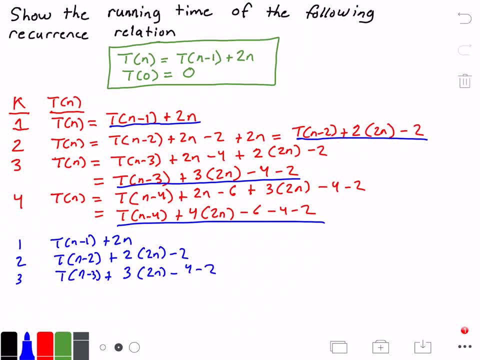 times n minus 4 minus 2.. And when k is equal to 4, we get t of n minus 4 plus 4 times 2 times n minus 6 minus 4 minus 2.. okay, so i'm going to erase everything that we did before. 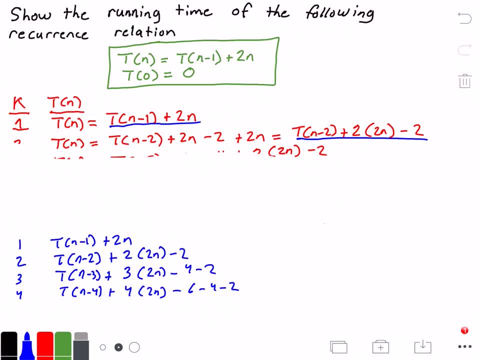 and hopefully now, uh, you guys can see a pattern as well. if not, i will try my best to explain. okay, all right, so here we have our k iterations and we have our function t of n. all right, so when k is equal to 1, we get t of n minus 1. when k is equal to 2, we get t of n. 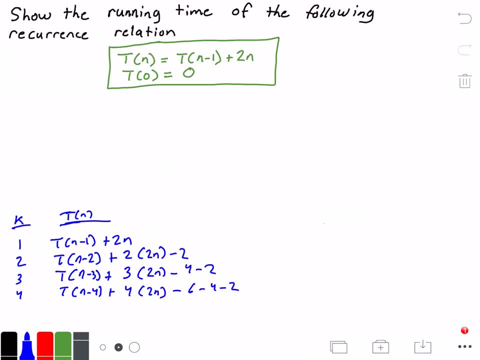 minus 2. when k is equal to 3, we get t of n minus 3, and when k is equal to 4, we get t of n minus 4. so we're trying to find a general form um for our problem here. so that general form. 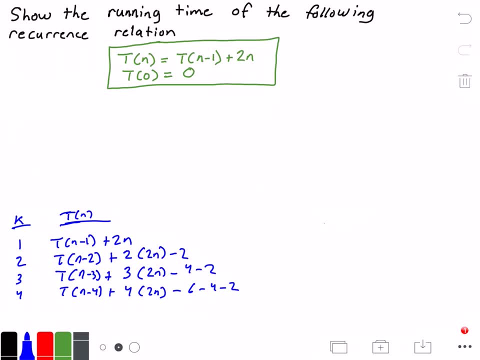 is. uh is basically what we is the equation that we see once we see this pattern. so for some arbitrary k value, so let's say that that we had, we were at iteration k, then our function t would look like this: it would be t of sorry here, t of n minus k right, and then, if i rewrite that first, um. 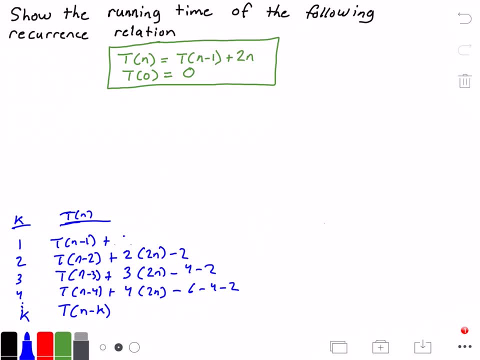 that first equation, so i can rewrite it to look like this, is still equivalent. so i have 1 times 2 times n, then we can see that this becomes k times 2 times n. okay, now for that last one. uh, that last step. here is it. i can see that it's a summation, actually. so 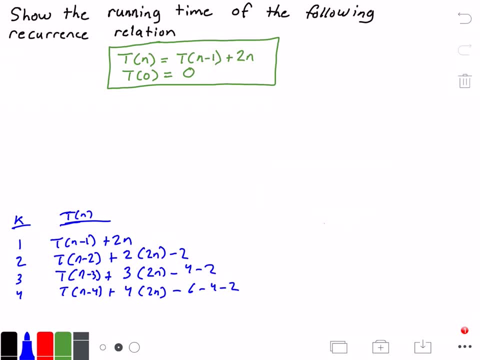 we're trying to find a general form for our problem here, So that general form is basically what we is the equation that we see once we see this pattern. So for some arbitrary k value, so let's say that we had, we were at iteration k- then our function t would look like this: It: 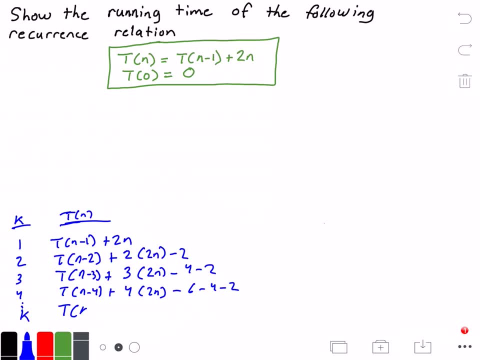 would be t of n minus 3.. And when k is equal to 4, we get t of n minus 4.. So we're trying to find a t of sorry here: t of n minus k, All right. And then if I rewrite that first, 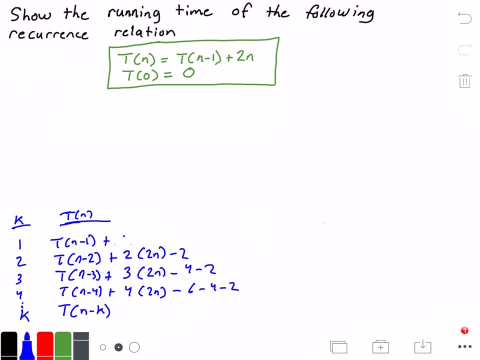 that first equation, so I can rewrite it to look like this: it's still equivalent. So I have 1 times 2 times n. Then we can see that this becomes k times 2 times n. Okay, Now for that last one. that last step here is: I can see that it's a summation actually. So 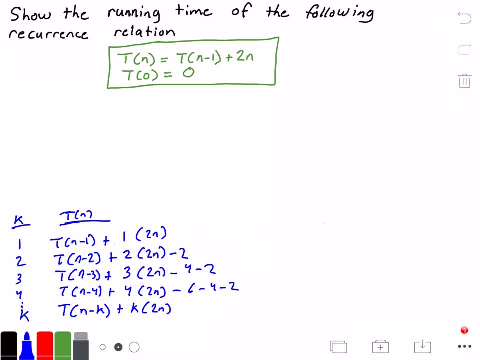 we can rewrite this equation as well. So we rewrite these equations we basically get. let me see: here I'm going to use the eraser. So for that second one you could think of it as a, as a minus 2 times 1.. For the next one: here you can think of it as: 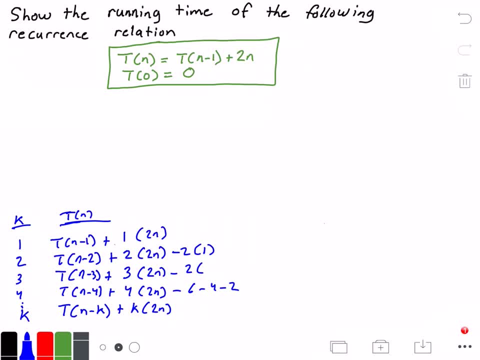 minus 2 times minus 2 times 2 plus 1.. And then that last one. if we rewrite it, we get minus 2 times 3 plus 2 plus 1.. And then here it will be, of course, minus 2 times. 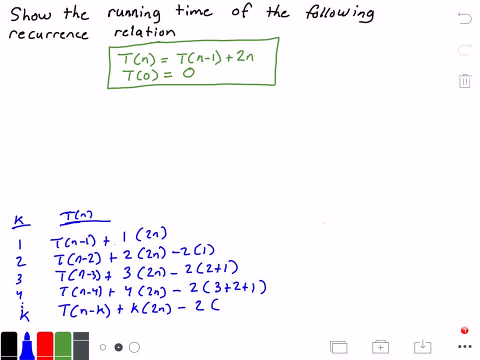 2 minus 2 times k minus 1 plus, k minus 2 plus, keep going down until we get to 1.. Okay, So that's just a summation, So the general form, and here I'll type or I'll write: general form. 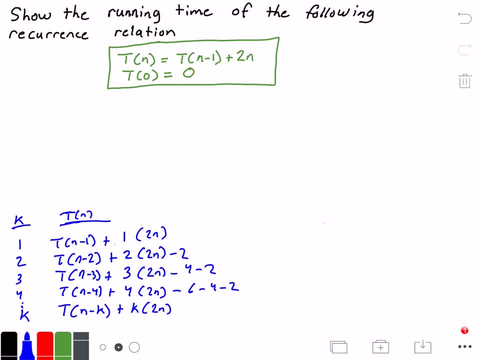 we can rewrite this equation as well. so we rewrite these equations. we basically get: uh, let me see, here i'm going to use the eraser. so for that second one, you can think of it as uh, minus two times one. for the next one here, For the next one here, you can think of it as minus 2 times 2 plus 1.. 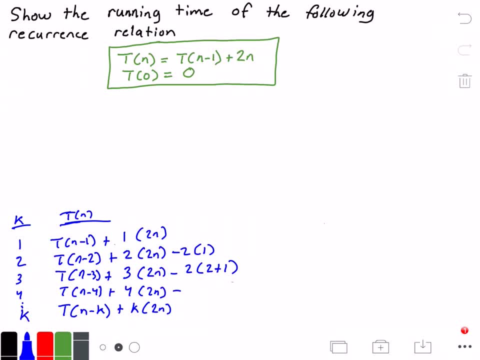 And then that last one. if we rewrite it, we get minus 2 times 3 plus 2 plus 1.. And then here it will be of course, minus 2 times 2, minus 2 times k, minus 1 plus k minus 2, plus keep going down until we get to 1.. 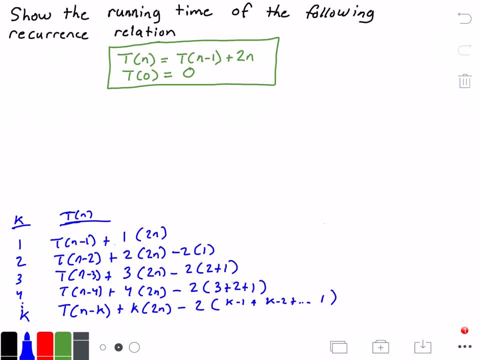 Okay, So, So, that's just a summation. So the general form- and here I'll type or write general form- is t of n minus k plus k times 2 times n minus. well, this right here is just. 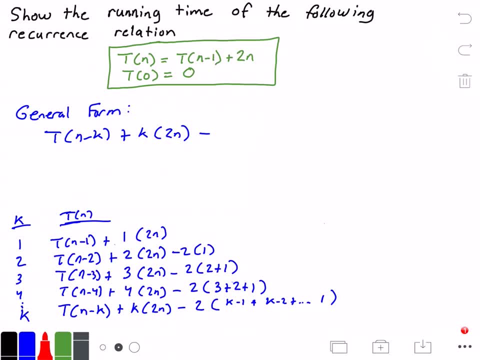 This is just a summation, And so we're going to write a summation here as well. So minus 2 times the summation from i equals 1, because that's where it stops, right all the way up to k minus 1.. 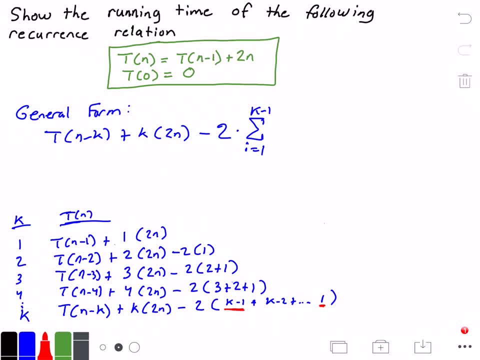 So we can see that it stops at 1, and we go up to k minus 1.. Okay, And this is going to be of i, All right, So let me go ahead and erase all of this that we've done now. 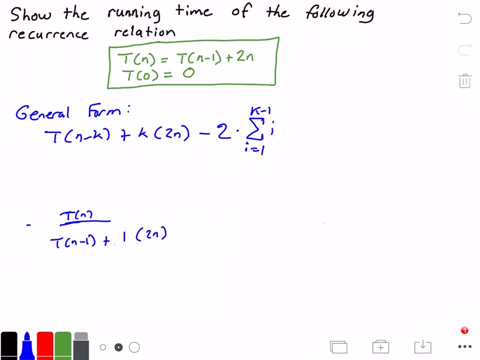 Hopefully I've explained it decently for you guys to understand. So now we have our general form and we need to know when this recursive case here is going to stop. So we need to get this whole form here, this whole general form in terms of n. 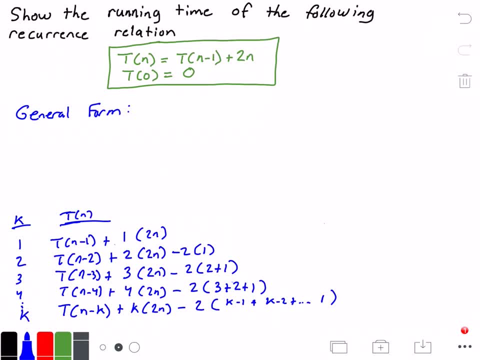 Is t of n minus k plus k times 2 times n minus. well, this right here is just a summation, And so we're going to write a summation here as well. So minus 2 times the summation from i equals 1, because that's where it stops right, All the way up to k minus 1.. 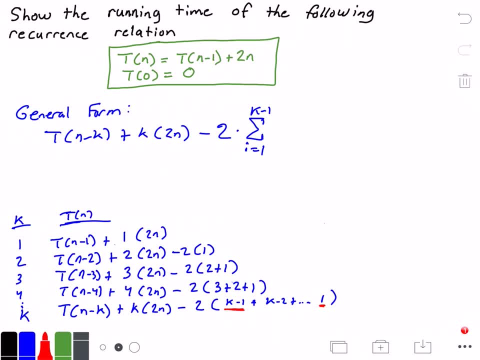 So we can see that it stops at 1, and we go up to k minus 1.. Okay, And this is going to be of i, All right, So let me go ahead and erase all of this that we've done now. Hopefully I've explained it decently for you guys. 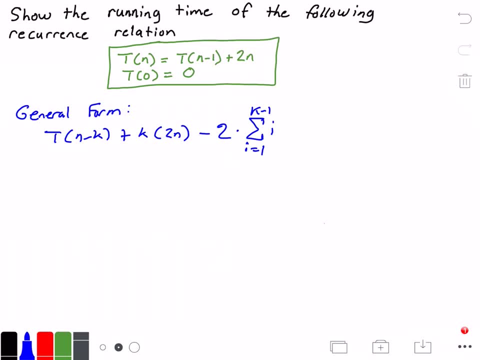 So now we have our general form and we need to know when this recursive case here is going to stop. So we need to get this whole form here, this whole general form in terms of n, And to do that we can just look at our base case. So our base case says that it's going to stop when n is. 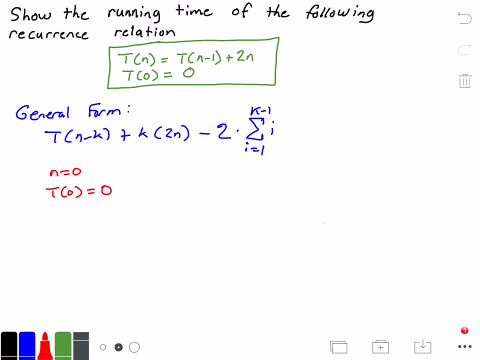 equal to 0, because t of 0 is equal to 0. So that means that we want t of n minus k to be equal to 0. And in order to do that, we need n minus k to equal to 0. And that means that n is equal to k, So we can substitute: 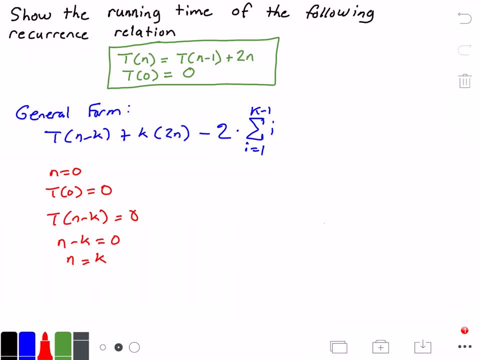 k for n and vice versa. So we want to get this in terms of n. So we're going to substitute out k for the value n. All right, Okay. Now if we rewrite our equation, we get t of n minus n plus n times 2 times n minus. 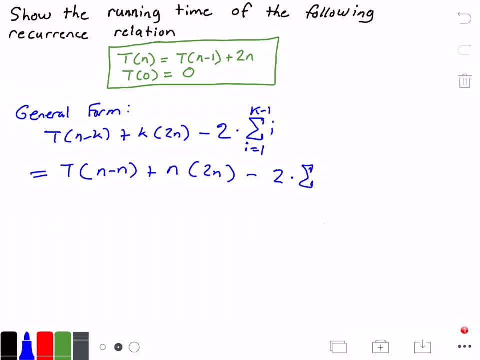 2 times the summation from n minus 1.. I'm sorry, from i equals 1 to n minus 1 of i. Okay, And if we rewrite this again, we get t of 0 plus 2 times n squared minus 2 times. 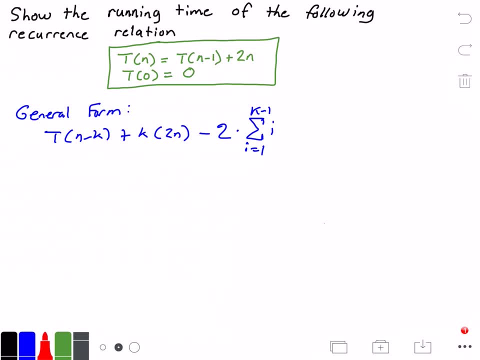 And to do that we can just look at our basis. So our base case says that it's going to stop when n is equal to 0, because t of 0 is equal to 0. So that means that we want t of n minus k to be equal to 0.. 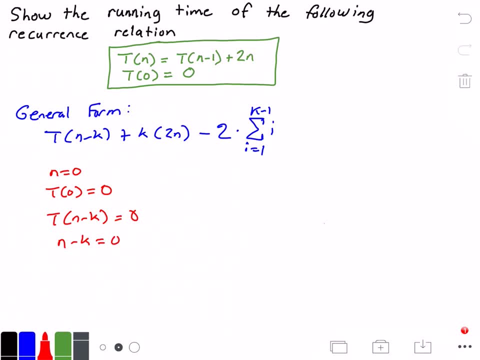 And in order to do that, we need n minus k to equal to 0. And that means that n is equal to k, So we can substitute k for n and vice versa. So we want to get this in terms of n, So we're going to. 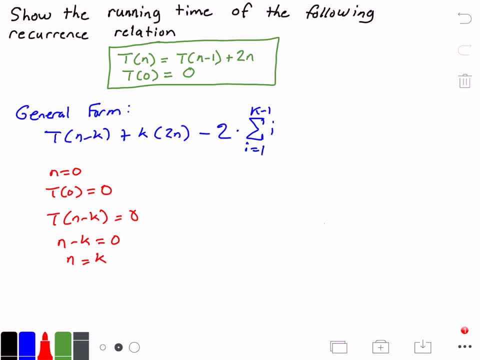 We're going to substitute out k for the value n. All right, So now if we rewrite our equation, we get t of n minus n plus n times 2 times n minus 2 times the summation from n minus 1.. I'm sorry, from i equals 1 to n minus 1 of i. 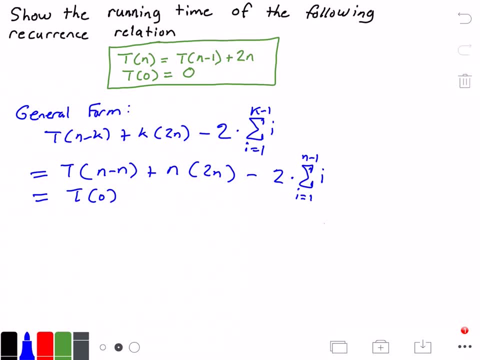 OK, And if we rewrite this again, we get t of 0 plus 2 times n. squared minus 2 times the summation from i equals 1 to n minus 1 of i. OK, And now we're going to rewrite this again. 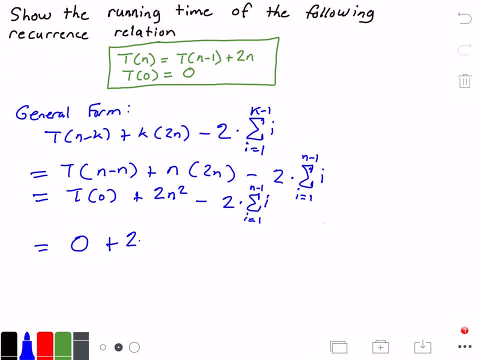 So this is equal to 0 plus 2n, squared minus 2 times. Well, let's actually solve for that summation, OK? So I'm going to put a little note here. So the summation from i equals 1 to n, minus 1 of i is equal to. 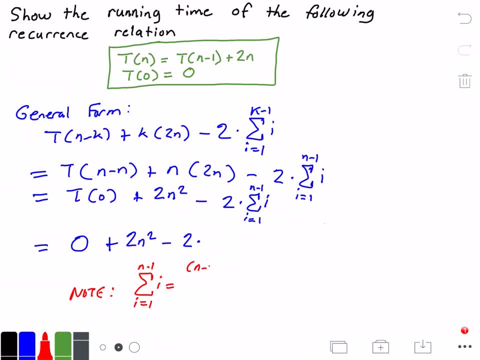 Let's see here: It's equal to n minus 1 times n divided by 2.. OK, How do I know this? Well, I remember a few. I have a few summation formulas, And one formula is this: So the formula that I'm actually remembering here is that the summation from i equals 1 to n, of i is equal to n times n plus 1 divided by 2.. 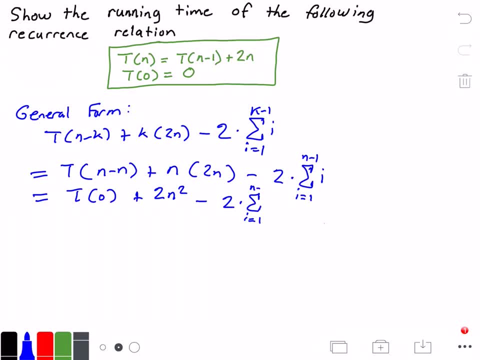 2 plus 1 is equal to n minus 1.. Okay, And now we're going to rewrite this again. So this is equal to 0 plus 2, n squared minus 2 times. Well, let's actually solve for that summation. So I'm going to put a. 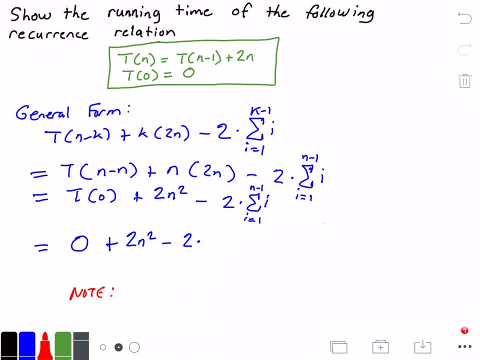 little note here. So the summation from i equals 1 to n minus 1 to n minus 2. I can just follow these items. make sure that I was at basically this right, Let's take a little note here. So the summation from i equals 1 to n minus 1, is equal to n plus 1 to n minus 2 this time. 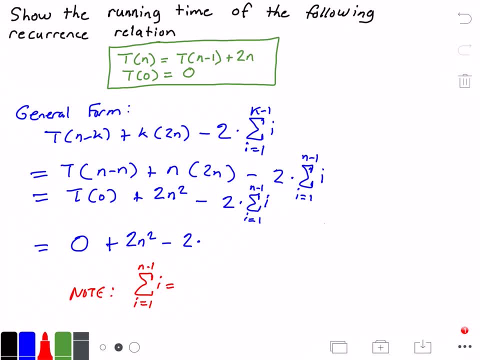 Submath, Submath, Submath, Submath, Submath, Submath. 1 of I is equal to. let's see here- is equal to n minus 1 times n divided by 2. okay, how do I know this? well, I remember a few summation formulas and one formula. 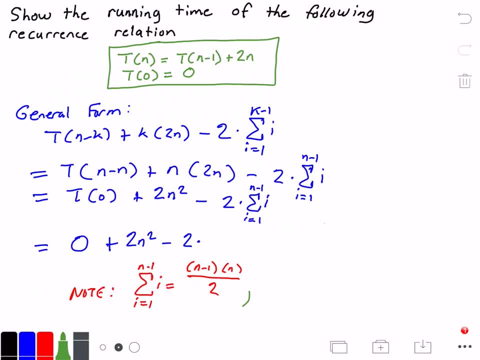 is this. so the formula that I'm actually remembering here is that the summation from I equals 1 to n, of I is equal to n times n plus 1 divided by 2, so I'm just substituting in n minus 1 into that formula. okay, all right, so let's go ahead. 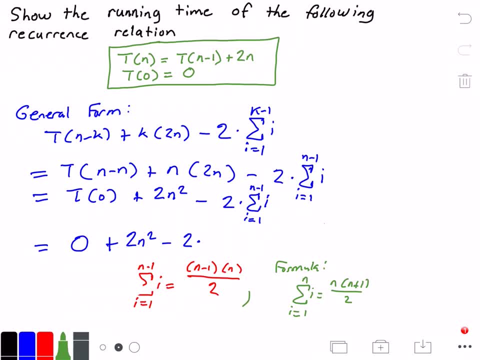 and get rid of this, get rid of all this here, and we're gonna put in that, that equation. now for our summation. so that is n minus 1 times n divided by 2. okay, so now, if we rewrite our equation one last time, we get two times in squared minus. let's see here: 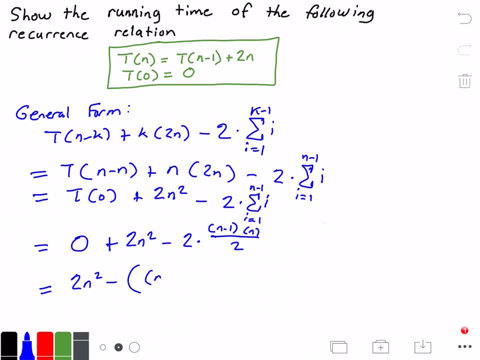 minus minus minus n, minus one times n, and that's because the two, the twos, will cancel out. all right, and i thought that that would be the last time, but look like we have to continue here. so this is equal to two times n squared. uh, let's see: minus n squared, minus n. 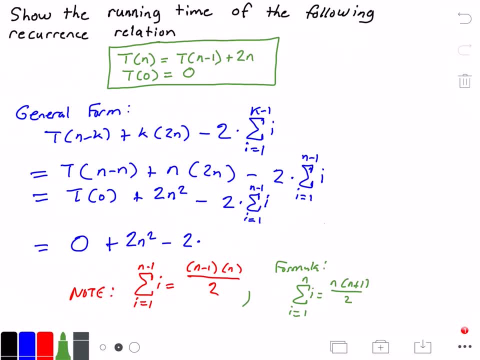 So I'm just substituting in n minus 1 into that formula. OK, So that's that, All right. So let's go ahead and get rid of this, Get rid of all this here, And we're going to put in that equation. now for our summation. 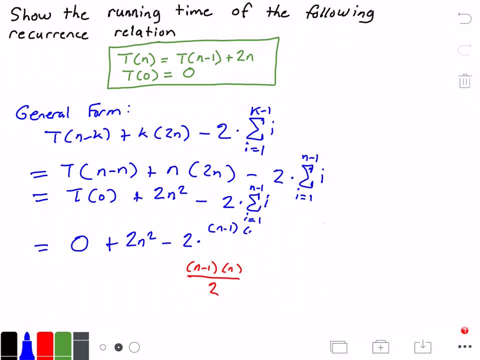 So that is n minus 1 times n divided by 2.. OK, So now if we rewrite our equation one last time, we get 2 times n squared. So there we go. OK, n squared minus. let's see here: minus n minus 1 times n. 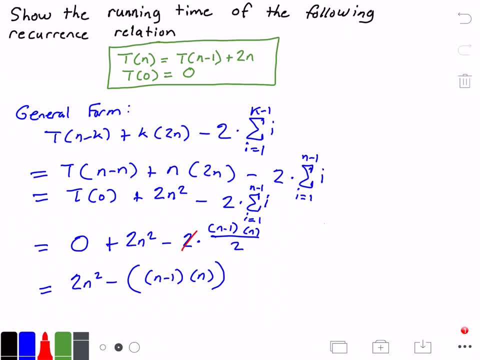 And that's because the 2, the 2s will cancel out. all right, And I thought that that would be the last time, but it looked like we have to continue here. So this is equal to 2 times n squared. 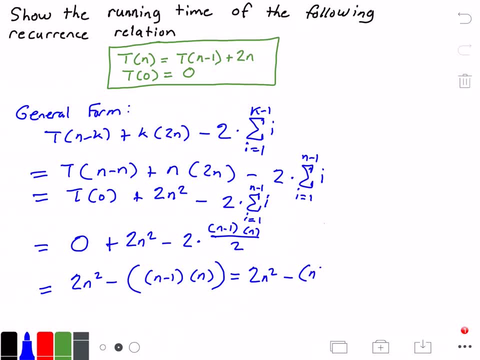 Let's see minus n squared minus n, And this is equal to 2 times n squared, minus n squared plus n- And I'm going to come down below here- And we get n squared, All right. so this is our guess of what this recurrence relation is equal to. 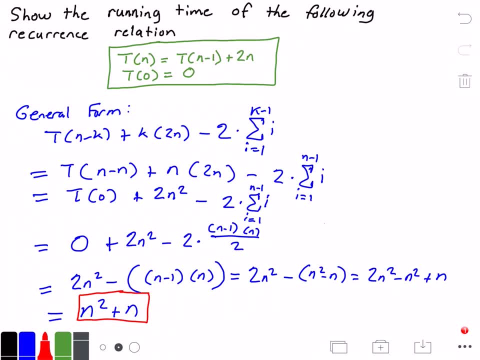 And this tells us that this is big O of n squared. Okay, So I know that was a lot of math, Guys. I hope you enjoyed this video. I hope it made sense. Please leave any questions you have in the comment section. 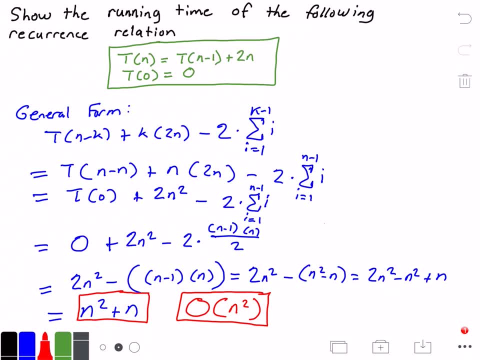 I'll try my best to get to you and answer the question. Please leave likes if you found this video helpful And please share it as well. That'll help me And it'll help others as well. So definitely click that like button and that subscribe button to subscribe to my channel for more videos like this. 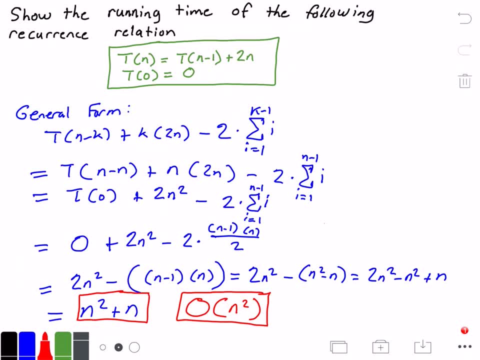